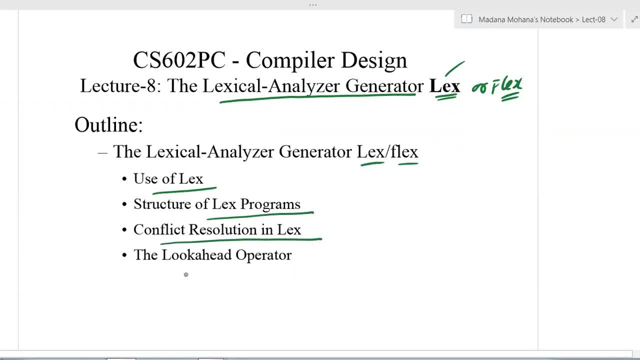 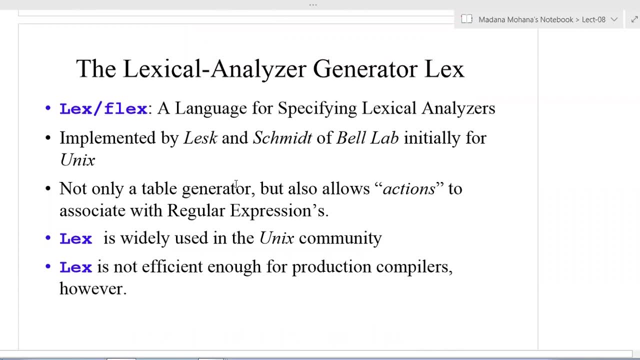 structure of a lex program, then some conflict resolution in lex, then the look ahead operator. Now coming to the introduction to lexical analyzer generator tool, lex or flex. So lex or flex, which is a long ways for specifying lexical analyzers, So implemented by two scientists. 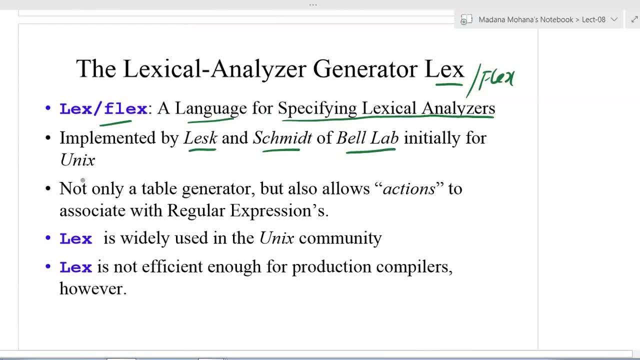 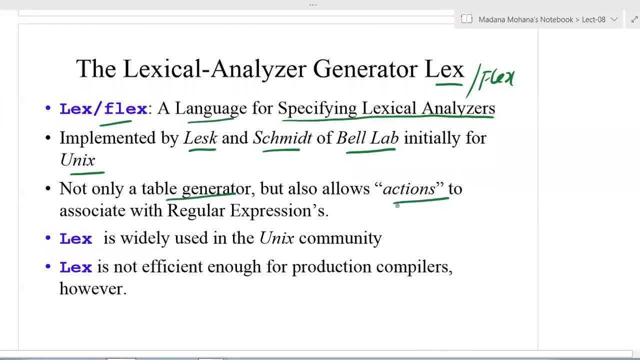 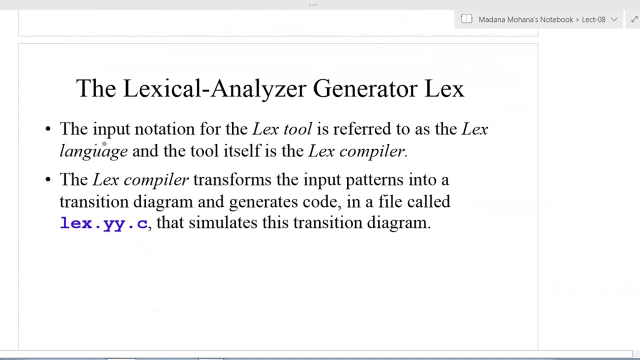 This tool not only a table generator but also allows actions to associate with regular expression. Lex is widely used in the Unix community. Lex is not efficient enough for production compilers, however, So alone lex is not efficient enough for producing new compilers. Then the input notation for the lex tool is referred to as the lex long ways. 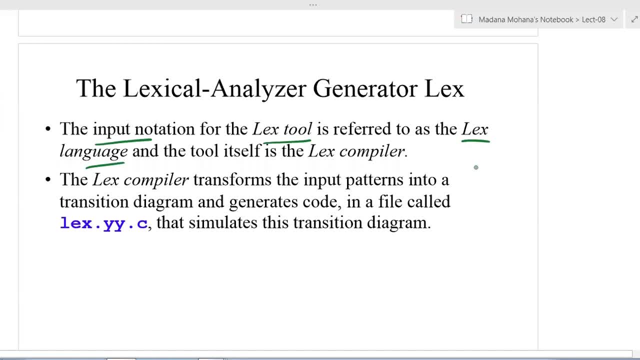 So the input notation for the lex tool is referred to as the lex long ways, So the input can be written in lex Longways with extension. This is the act matinfor lex programming longways. Then the tool itself is considered as a lex compiler. The lex compiler transforms the 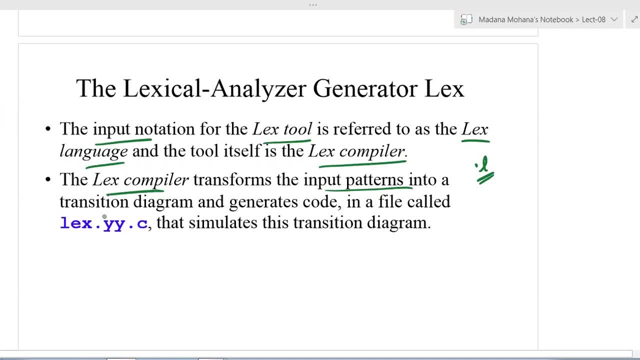 input patterns into transaction diagram and generates code in a file called lexya. This is the C file. dot hade extinct. is the C programming language Here. lex, then ya value. VL is 1. là la valence. ça depend. have un rupture dans le textフ. statopp, TypeX, then yy value. 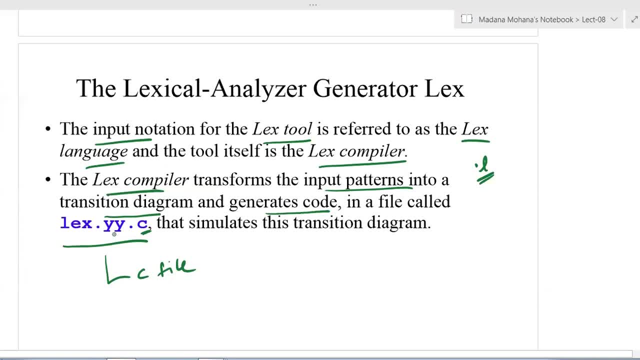 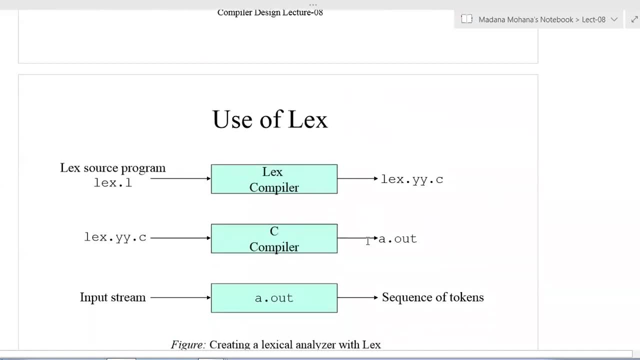 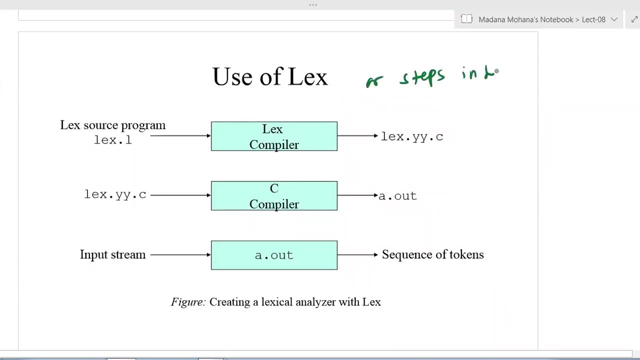 value is the one of the command which gives this value to the parser letter, so which simulates this transition diagram. now let us see the use of flex, or steps in flex implementation. so here we have three phases or three steps. first, the input can be written in lex language source program. 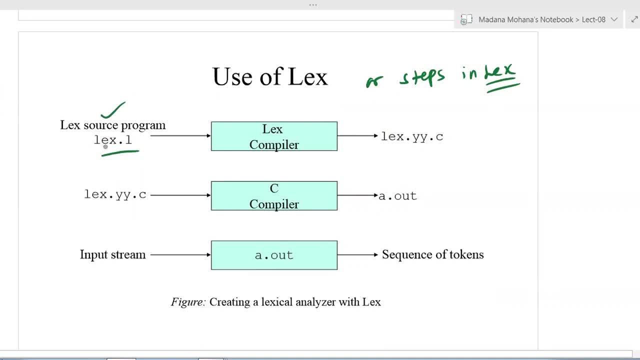 with extension dot l, lex dot l. here, whatever the file name with extension dot l you have to give, then using lex compiler this can be converted into c programming language, that is c language code. so lex dot yy, dot c. then this c language code is converted into object code using c compiler. 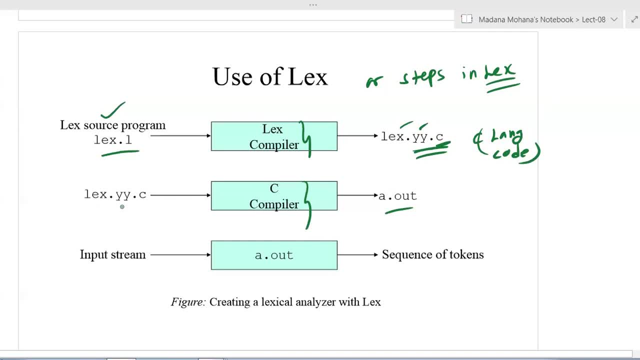 okay, the input of the c compiler is this one source program in c, x, dot, yy, dot, c. then uh, by using c compiler this can be converted into object code, a dot out, which is called as object code. now this object code further takes input stream, then produces sequence of tokens. so finally, 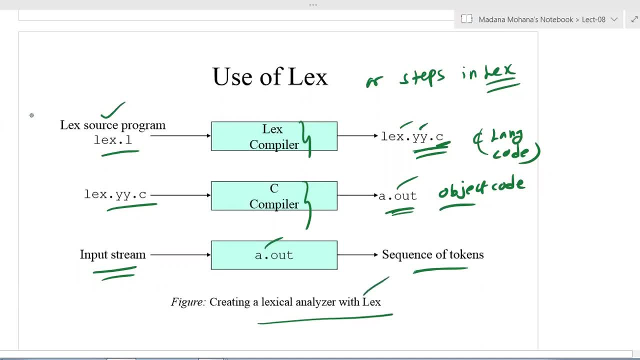 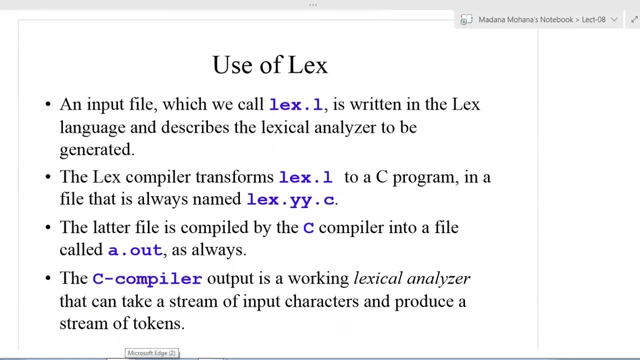 this figure shows creating a lexical analyzer using lex tool with the three pages or three steps: one, two, three, then explanation about the previous diagram. an input file, which we can call lex dot l, is written in the lex language and describes the lexical analyzer to be generated. then the lex compiler transforms lex dot l to a c programming language into a file that is always. 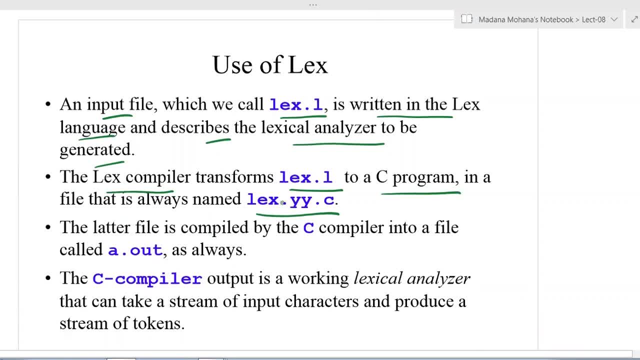 named as x, dot, yy, dot c, so on the standard predefined names we have to use same only, irrespective of whatever the file name. the latter file is compiled by using c compiler into a file called a dot out, as always, then the c compiler output is a working lexical analyzer. 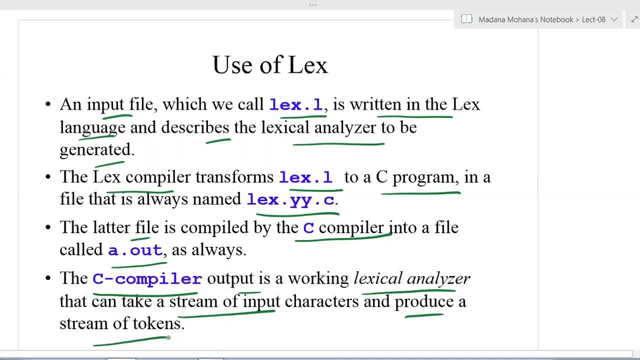 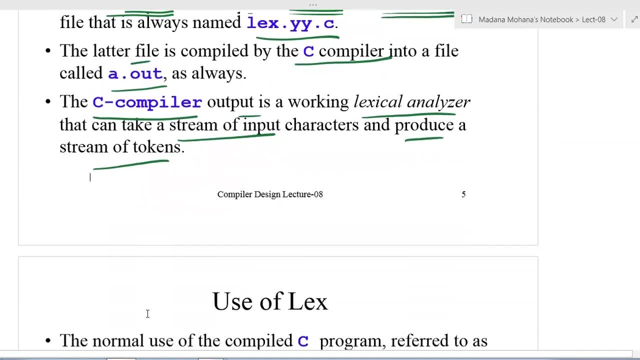 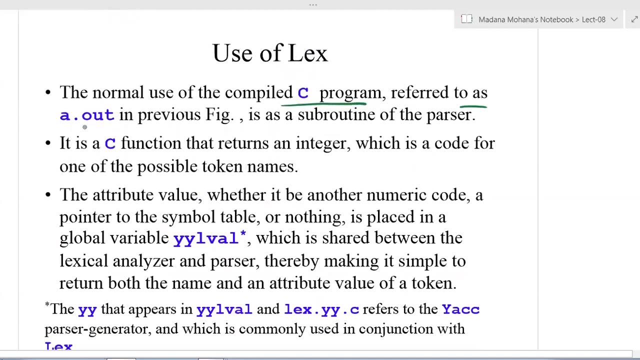 that can take a stream of input characters and produce a stream of tokens. that is, a dot out takes input as input stream, then produces stream of tokens. so then the normal use of the compiled c program referred to as a dot out in the previous figure, what we mentioned is a subroutine of the 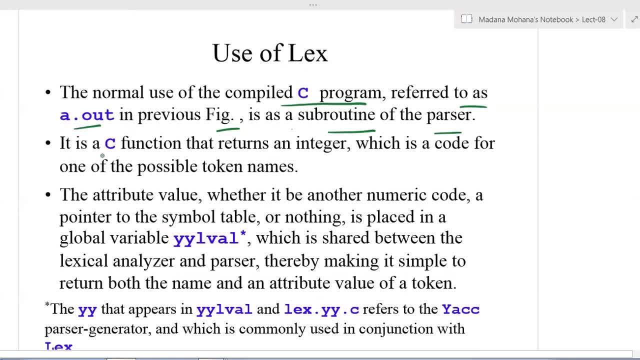 parser or syntax analysis. it is a c function that returns an integer which is a code for one of the possible token name. the attribute value, whether it be another numeric code, a pointer to the symbol table or nothing, is placed in a global variable: y y l value. so what is y y l value? this is a global. 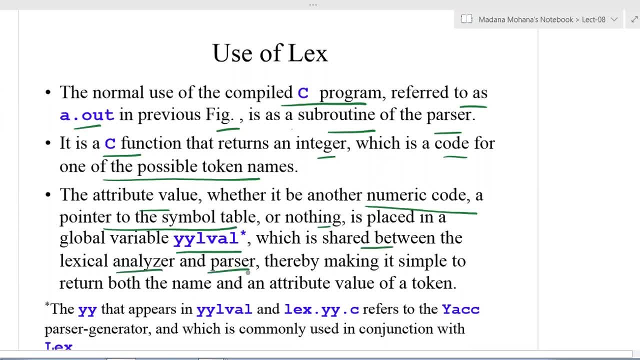 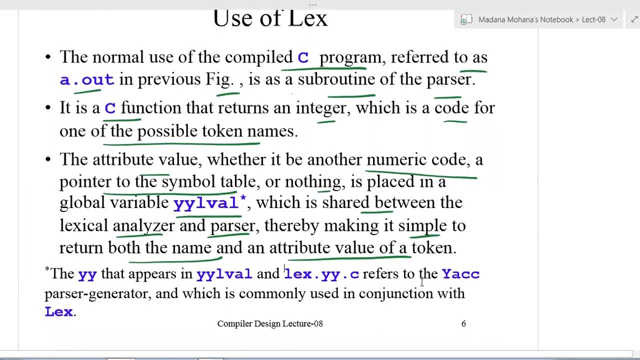 variable so, which is shared between the lexical analyzer and parser, so innocent, to symbol table. we can use y, y, l value, so which shows the interaction between lexical analyzer and parser there by making it simple to return both the name and attribute value of the token. actually, the name and attribute values are stored in the symbol table, so earlier, without 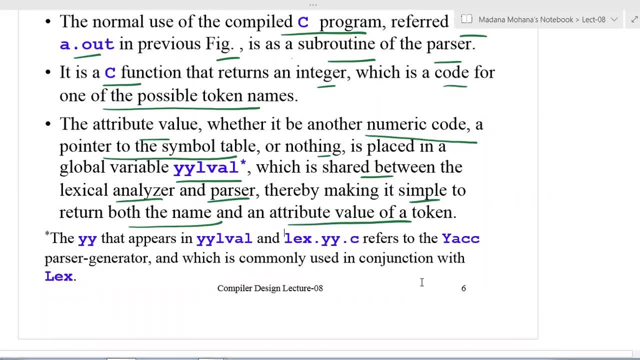 symbol table, also globally, by using the variable y y l value. this can be done. so here the y? y that appears in y y l value and lex dot y y dot c refers to the parser generator, which is called as yacc. in the next phase of compiler, that is, syntax analysis of parser, we will discuss about this. 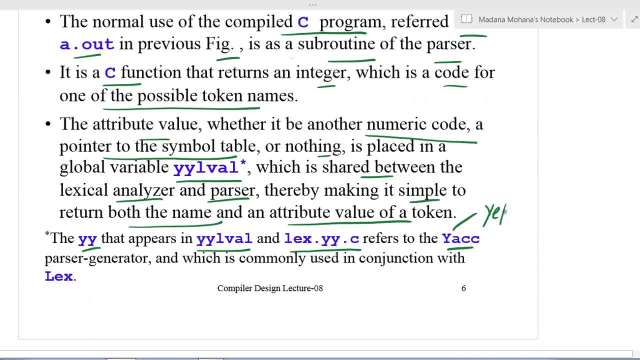 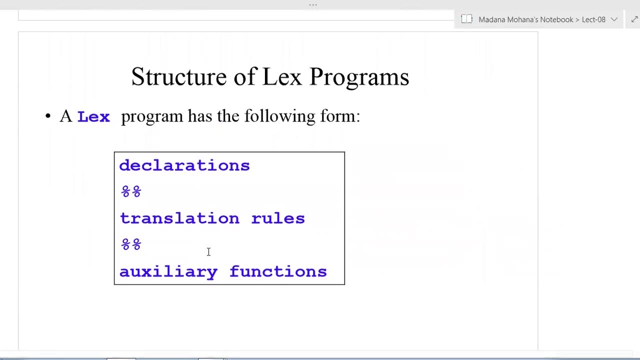 automatic parser generator, which is called as yacc, at another compiler compiler- this is the abbreviation for yacc, compiler compiler, so and which is commonly used in conjunction with lex tool. they are coming to structure of lex program. so lex program, consisting of three steps, are three parts. the first part is declarations, so can be defined. 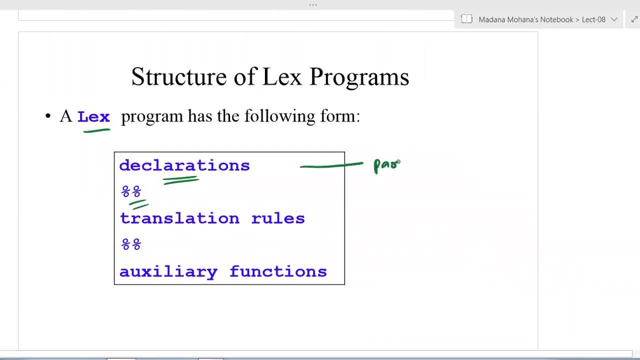 defined using percentage symbol. so this is part one of the lex program. then second part, called as translation rules. here we will define the definitions of regular expressions for the tokens. this is part two. here we will define definitions of tokens. that means rules. then this, also defined using the delimiters percentage symbol. then part three, which is called as: 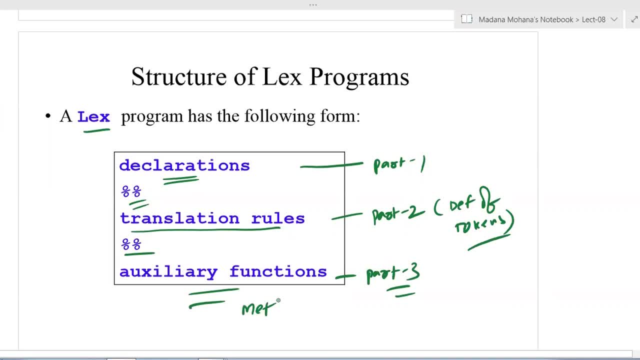 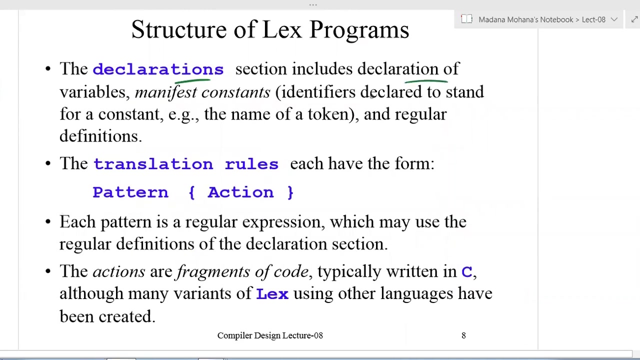 axillary functions. here methods are additional functions are defined. these are all the three parts of lex program. now let us see one by one with example. first section, The declaration section, include the declaration of variables, manifest constants, like identifiers, declare to stand for a constant, example, the name of the token and regular definitions. 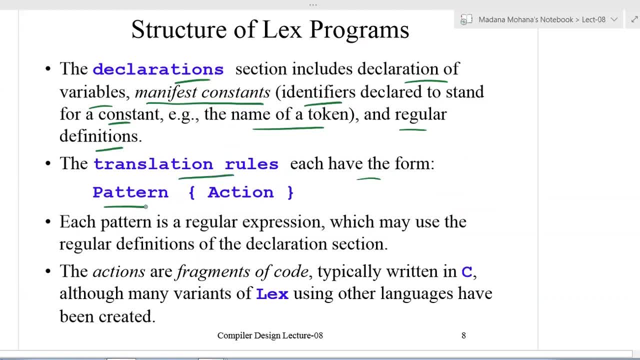 Then the translation rules each have of the form, the pattern, followed by action, what it returns. Then each pattern is a regular expression which may use the regular definitions of the declaration section. Actions are fragments of code typically written in C language, although many variants of lex. 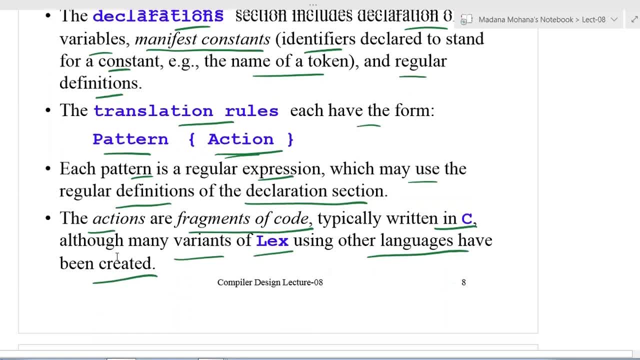 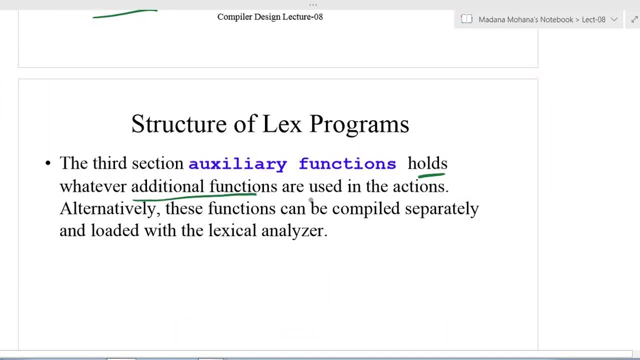 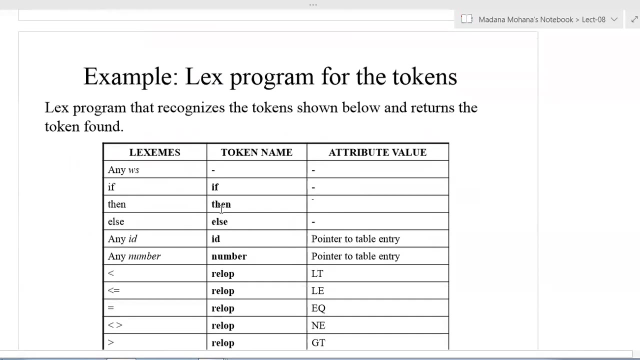 using other languages have been created. Then the last section, auxiliary functions, which holds whatever additional functions are used in the actions. alternatively, these functions can be compiled separately and loaded with lexical analyzer. These are all the three parts of lex program. Now let us see one example program. 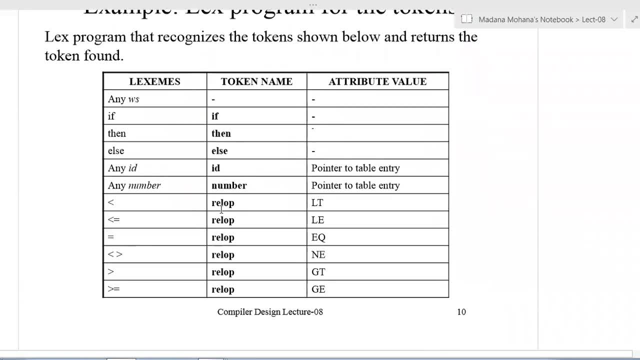 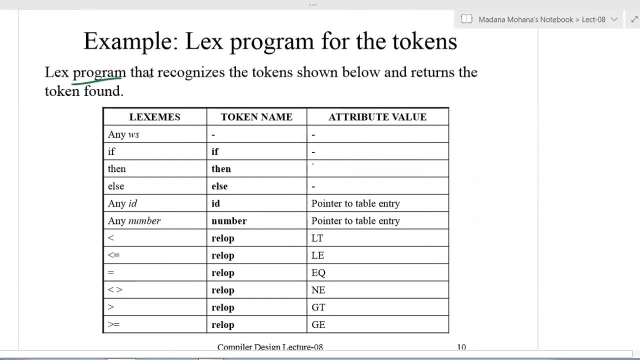 So this token example we already covered in our previous lectures. for this we will see how the lex program is implemented. Lex program that recognizes the token shown below and returns token is formed. The output of lex program is: a particular token is formed. The table consisting of lexin token name, attribute value. 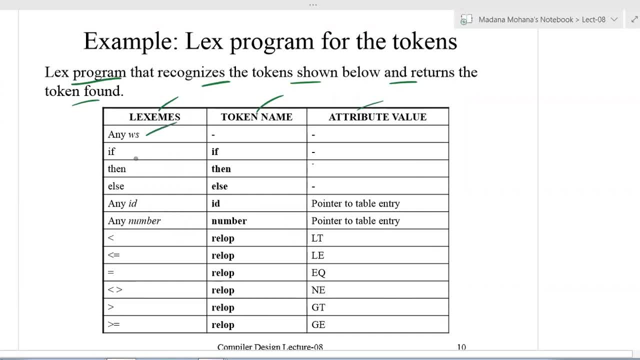 In the previous lecture we discussed same table, Widespace, Then the keyword, if, then else, then identifier id number, then relational operators: less than less than or equal, equal, not equal, greater than greater than or equal. 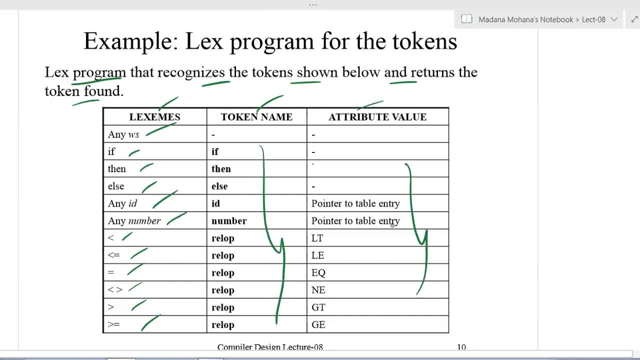 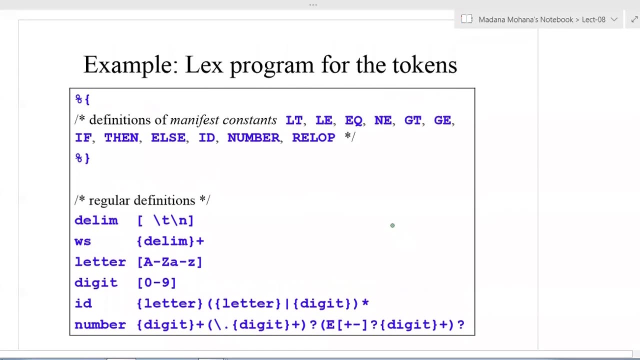 The tokens, as well as attribute values, are shown in this table. Now, all these we are going to define in the lex program in the part of declaration and translation rules. Then let us see the lex program for this token. So first section, Okay, 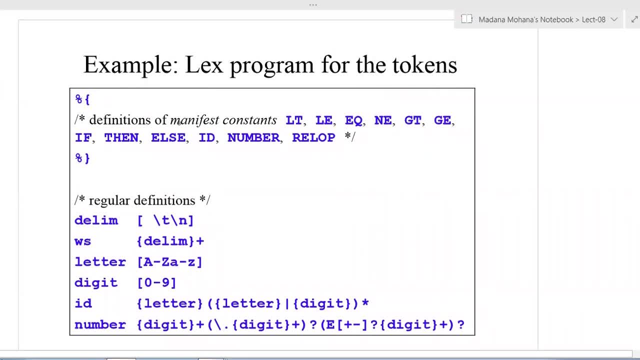 Here, first, we will define all the constants, manifest constants used in the previous example: less than less than or equal, equal, not equal, greater than greater than or equal. If then else keywords, identifier, id number, then relational operator or LOP. 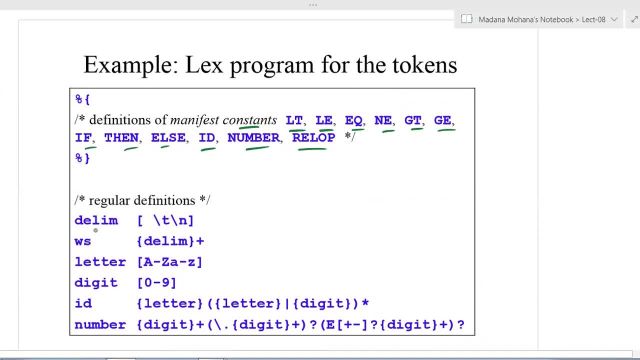 These are all manifest constants, Then regular definitions for all these tokens. regular definitions: Delimiter can be defined as space, followed by tab, followed by new line, Then widespace. This is nothing but delimiter with repetitions excluding null positive closure. 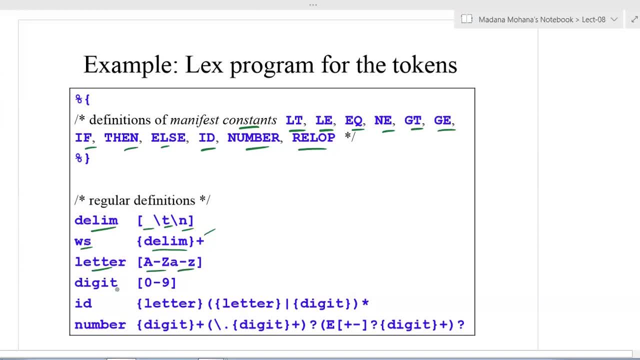 Then letters: uppercase combinations a to z. lowercase combinations small a to z. Then digit 0 to 9.. Then identifier: definition: letter followed by letter or digit: whole closure. Then number: unsigned number: The definition is digit positive closure. 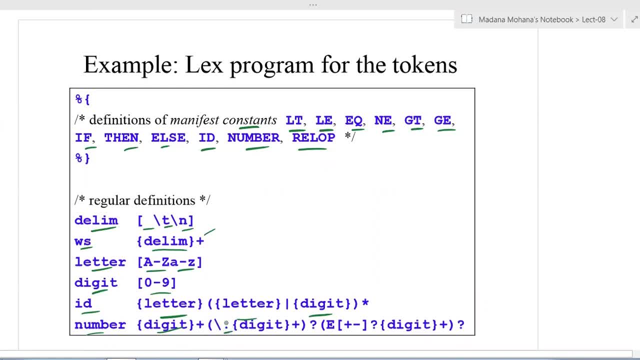 Then widespace slash, then floating point, then again digit. positive closure, then question mark. Positive or negative exponent value then question mark, then digit. whole closure, positive closure, then question mark. So these are all the regular definitions of all the tokens. 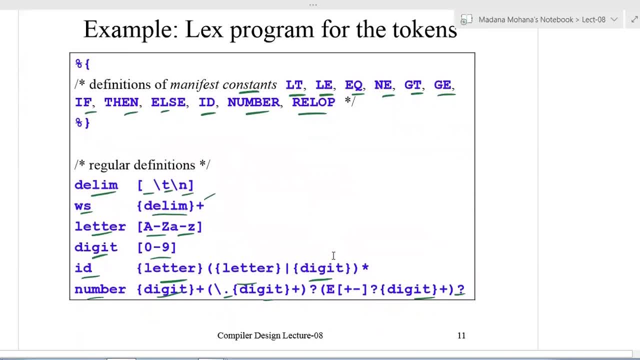 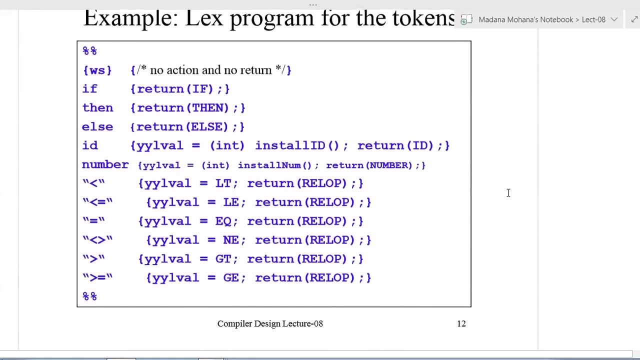 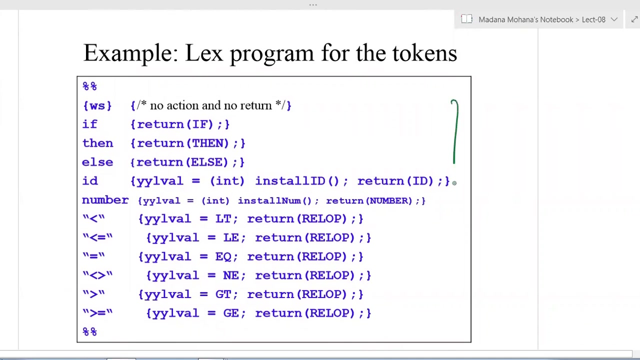 Now this part is called as declaration part. This part is called as declaration part. Now the second part is declaration part. Okay, The second part: translation rules. here we will define all the actions of the tokens defined in the previous section. So this part is called as translation rules. second part. 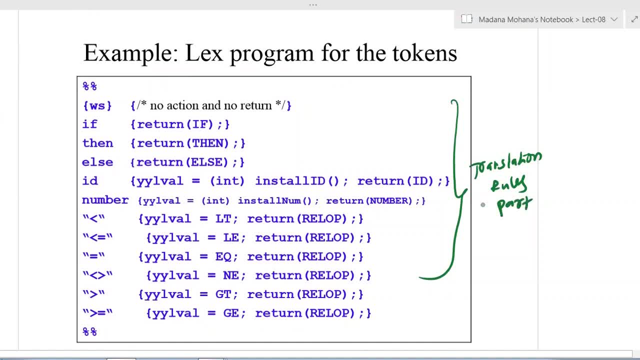 Translation rules part. So here all the tokens: what we defined in the previous section, now those actions are defined here. That means first, whenever widespace is found, Okay, Now it will return no action. It returns no action, no return. Whenever the keyword if is found, it returns if. 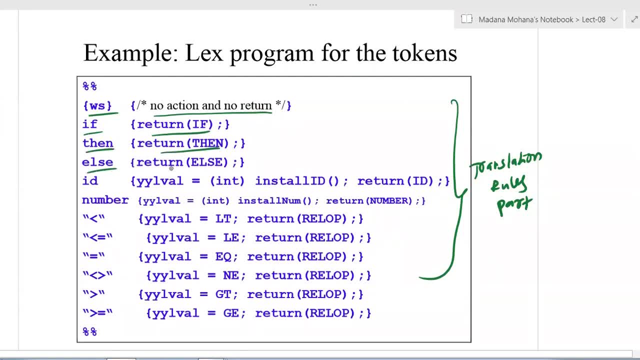 Whenever the keyword then is found, it returns. then. Whenever the keyword else is on, it returns else. Whenever the keyword identified is found, it returns yylvalue equal to it. calls of method: install id and return id. These are all the two methods. 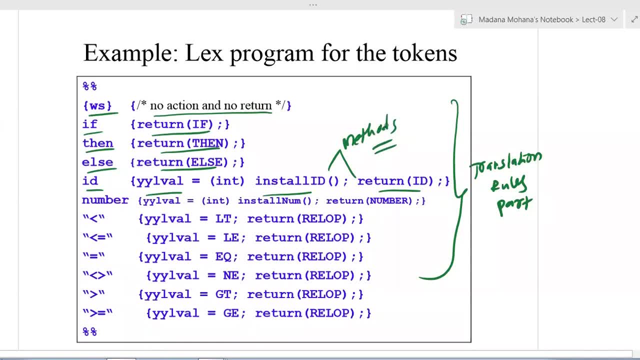 What are the methods are defined in actions, So these methods are implemented in the next section, that is, auxiliary functions. their number calls yyl, value equal to it calls the method install number. then returns number. both methods type is integer. then whenever it sees less than symbol, it calls yyl equal to lt, the attribute. 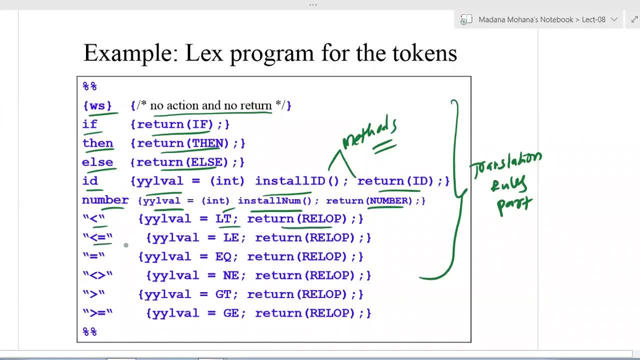 value lt. returns the token name as relational operator, then less than or equal. it returns le. returns rel op, then equal. it returns eq, then not equal. it returns ne as a relational operator, then greater than. it calls the attribute value gt, then returns rel op, then greater than or equal. 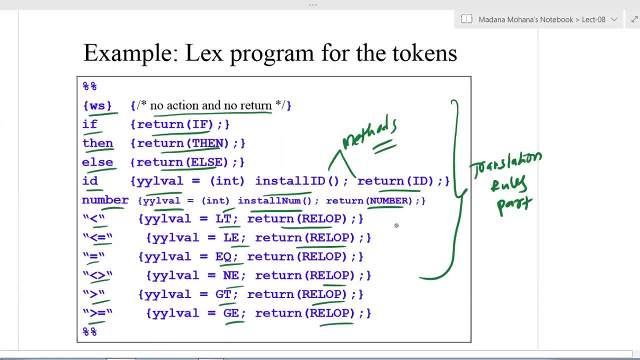 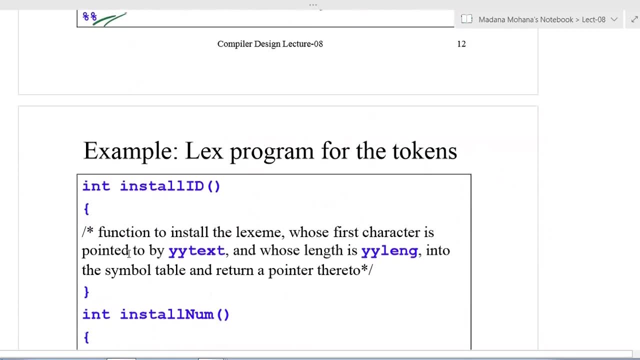 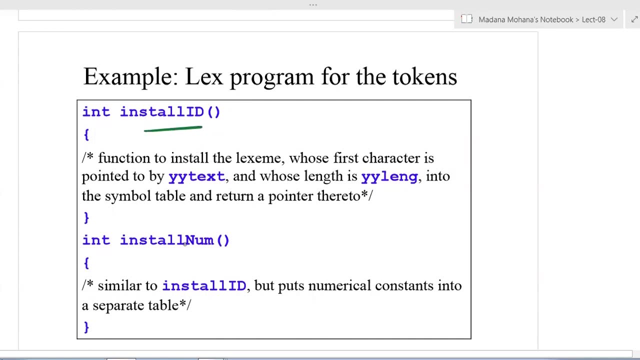 it returns ge, then returns rel op. now, all these are all defined between the delimiter double percentage symbol. then, coming to the last section, that is, translation functions, in the actions of the previous section two methods are used, that is, install id and install number. those methods are implemented here under auxiliary function. so this is the third part, auxiliary. 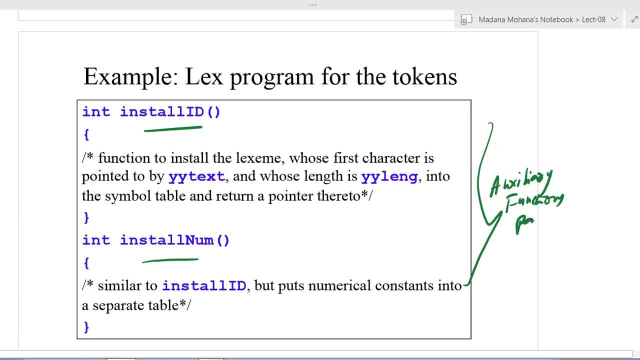 functions. functions part of the lex program. the first one: int install id. this function to install the lexim whose first character is pointed by two variables, that is, yy text and whose length is yy, len g into the symbol table and returns a pointer there too, using these two variables. those can be: 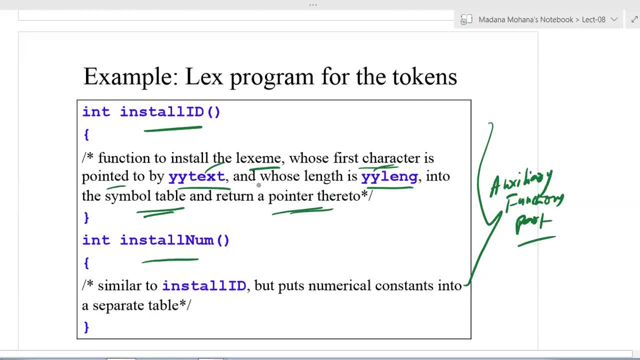 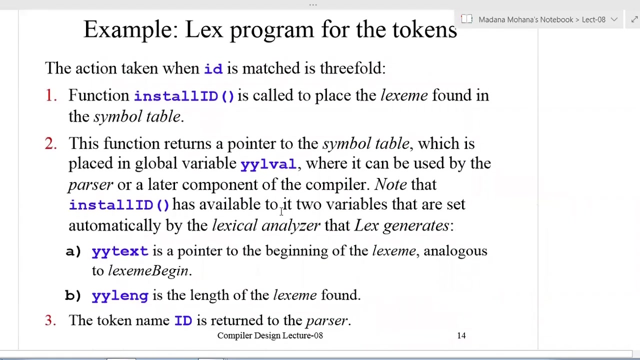 stored into symbol table and returns a pointer to the to those variables. then, second method: install number similar to the install id but puts numerical constants into a separate table. the information about identifiers and numbers are stored in the symbol table using these variables: yy text and yy length for identifiers. here some of the actions are different. 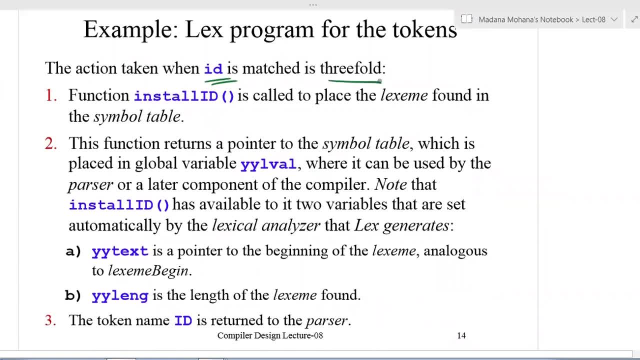 the action taken when identifier is matched is a threefold with three cases. the first case: the function install id is called to place the lexim found in the symbol table table. whatever we mentioned in this, This function returns a pointer to the symbol table which is placed in global variable yyl value where it can be used by the parser or syntax. 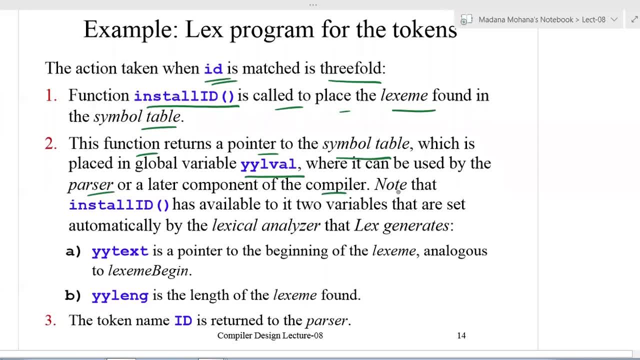 analysis or the latter component of the compiler. Here one of the note that install id has available to it two variables that are set automatically by the lexical analyzer that lex generates. What are the two variables? yytext and yyl length. yytext is a pointer to the beginning. 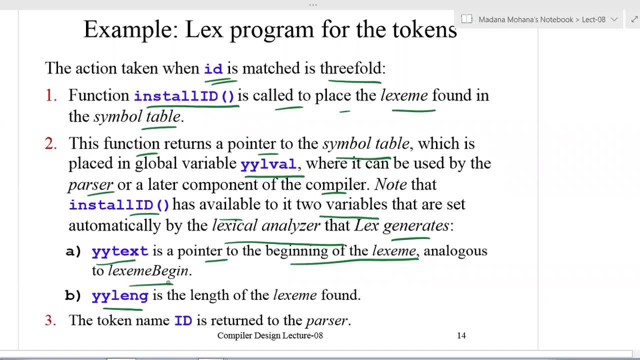 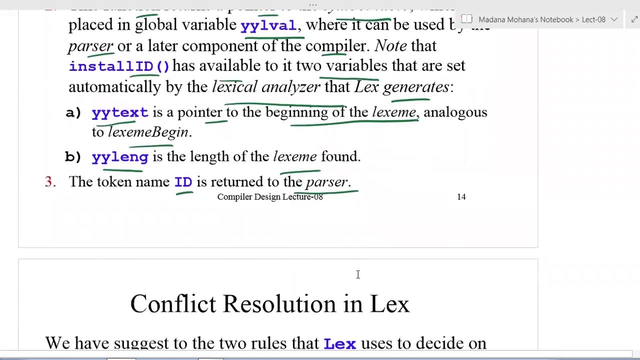 of the lexem which is analogous to lexem begin. Then yylength is the length of the lexem found. Then the third point is the token name id is written to the parser, which is the next phase of the compiler, also called as syntax analysis. 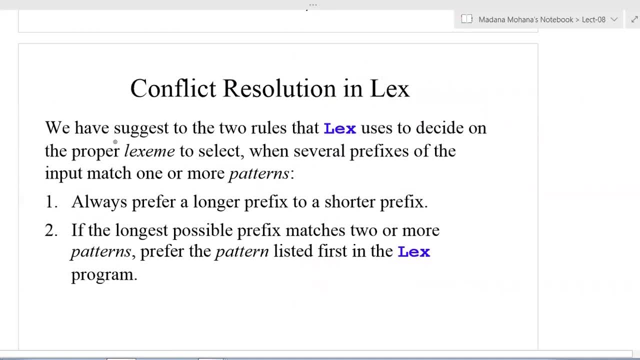 Then coming to conflict resolution in lexer. So here this can be handled In the following way: we have suggested to the two rules that lex uses to decide on the proper lexem to select when several prefixes of the input match one or more patterns, The 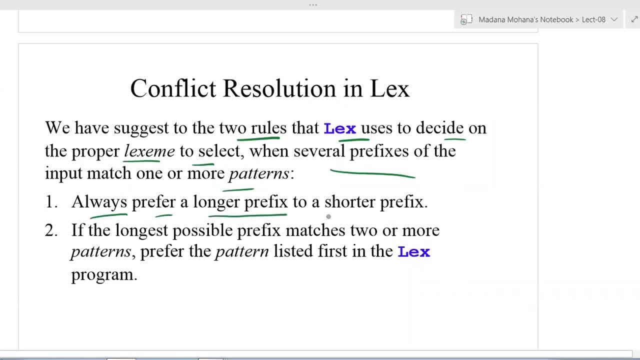 first rule is always: prefer a longer prefix to a shorter prefix. So whenever longer prefix is given, then you can convert into shorter prefix. that can be considered. And if the longest possible prefix matches two or more patterns, then prefer the pattern listed in the lex program which is considered here. So, using these two rules we have to overcome. 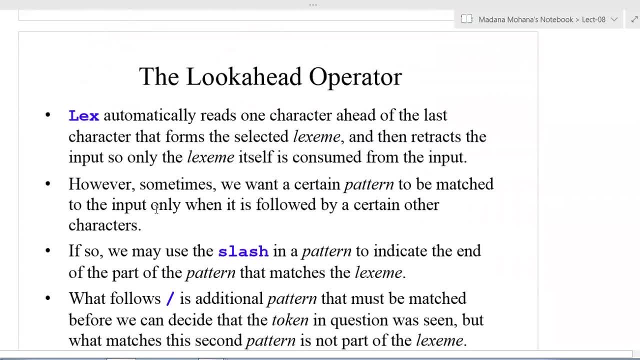 the conflict resolution in lex. Then, coming to the lookahead operator, The lookahead operator in the input buffering can be implemented using lexem begin and forward pointer. The same thing, so how this can be done in lex program. So lex automatically reads one character ahead of the last character that forms the selected. 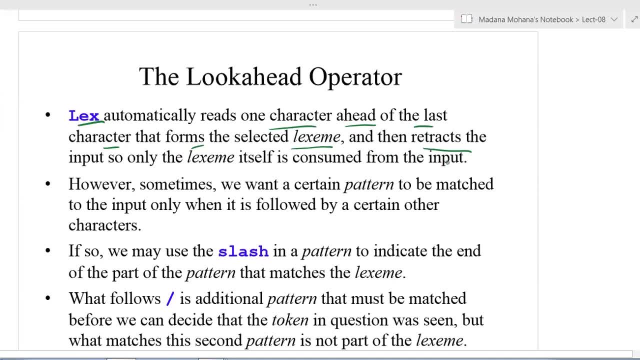 lexem and then retracts. that means one position moves ahead. that is nothing but a retract. So retracts the input, so only the lexem itself is consumed from the input. however, sometimes we want a certain pattern to be matched to the input only when it is followed by a certain 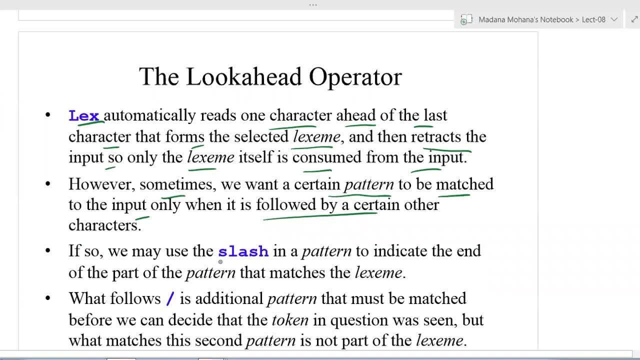 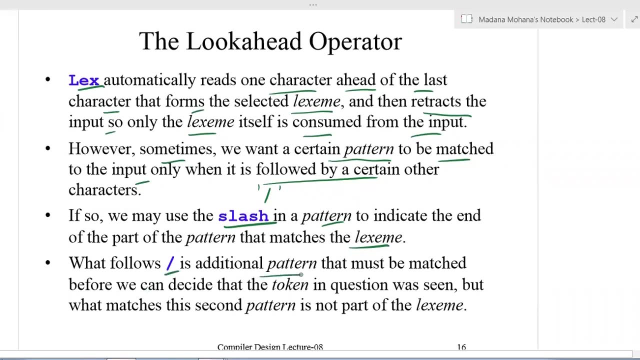 other characters here. this can be done by using slash symbol in your pattern to indicate the end of the part of the pattern that matches to the lexem. So what follows slash is a additional pattern that must be matched before we can decide that the token in your question was seen. but what matches the second pattern is not part. 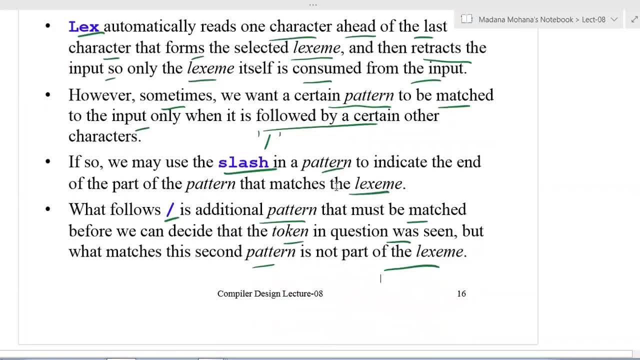 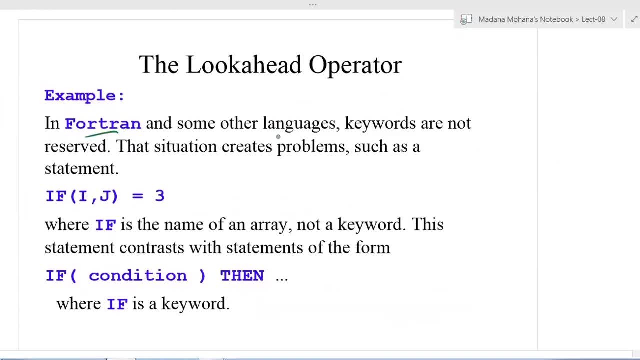 of the lexem. So like this. So this can be implemented. Let us see one example for this implementation. in Fortran language and some other languages, keywords are not reserved in this case. this situation creates a problem, such as the statement: if i comma, j equal to 3. here you can see the Fortran and other languages not recognizes. 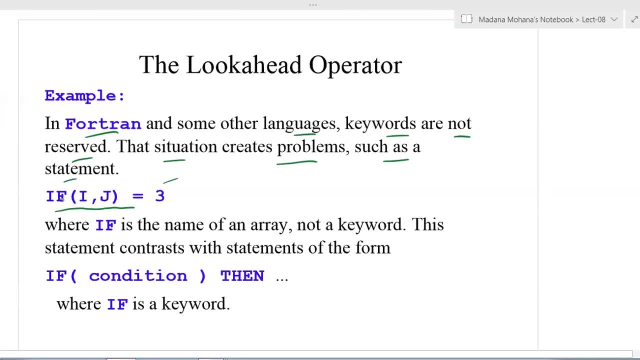 the keywords. So now this can be implemented. This can be treated as if is. it can't be identified as a keyword because it can't result. So in this case now, where if is treated as name of the method called array, so it is not. 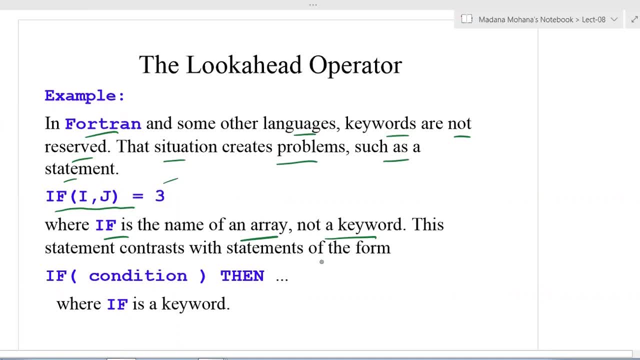 a keyword, So this statement contrasts with the statement of the form. the same statement can be translated into here. you can see if condition, then Now this looks like this is a conditional statement here, where if is a keyword or there's a difference between these two statements. 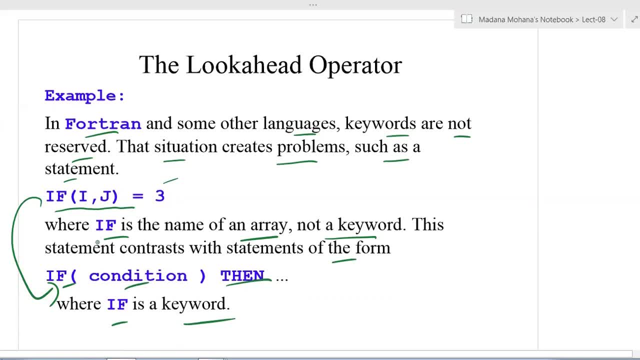 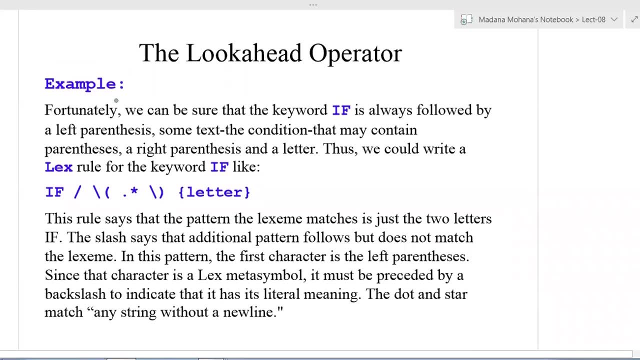 These type of situations can be handled by using lookahead operator. how this can be converted into recognizable form, here you can see. So fortunately we can be sure that the keyword if is always followed by left parenthesis, then some text, Then the condition that may contain parenthesis, then a right parenthesis and a letter. 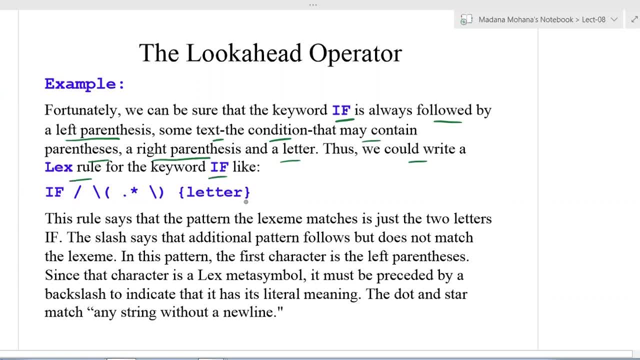 Thus we could write the lex rule for the keyword if like this: so if slash, then followed by backslash, then parenthesis, then dot asterisk, then backslash, then right parenthesis, then the action letter. Here What it means. What it means, What is the meaning of this rule? 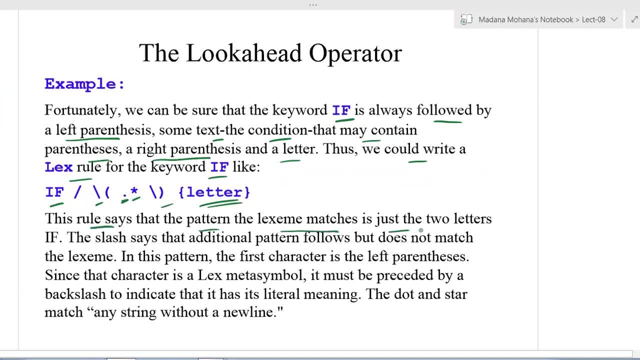 This rule says that the pattern the lexium matches is just the two letters, i and f. The slash says that additional pattern follows but does not match the lexium. In this pattern, the first character is the left parenthesis- left parenthesis this one, since the character is a lex meta symbol about the data data, about the data it must be preceded. 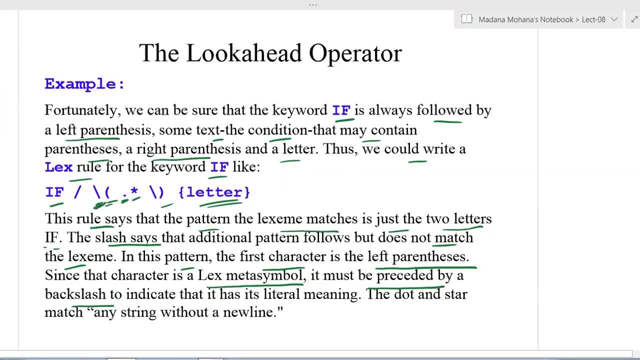 by a backslash. This one backslash meta data to indicate that it has literal meaning that dot and star matches the dot and star matches any string without a new value. This has an explanation of each and every symbols occurred in this rule. So this is the lex rule for the keyword. if like that, we will implement the lookahead operators. 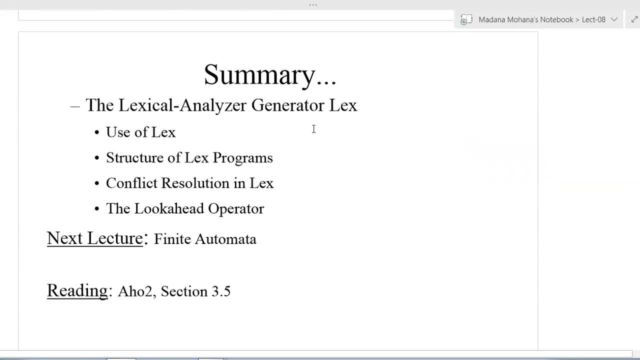 to avoid the conflicts. So Now coming to summary of this lecture, in this lecture we covered lexical analyzer generator, lexor flex: introduction, followed by use of the lex with the various pages, then structure of the lex program with the example program is demonstrated. example program, then a conflict.